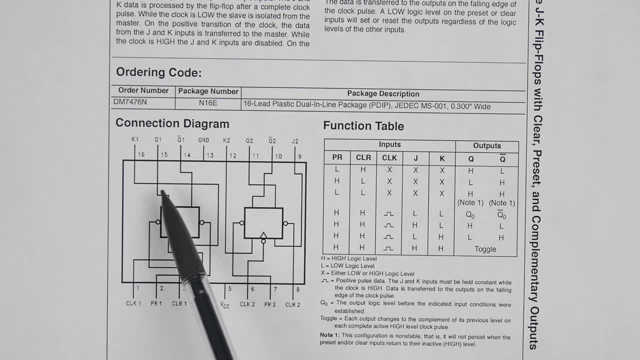 And there's other chips that have JK flip-flops- the 74LS73 I think, and yeah, I think pretty much anything you find that claims to be a JK flip-flop. if you've got the datasheet, you should probably be able to figure out how to set it up. 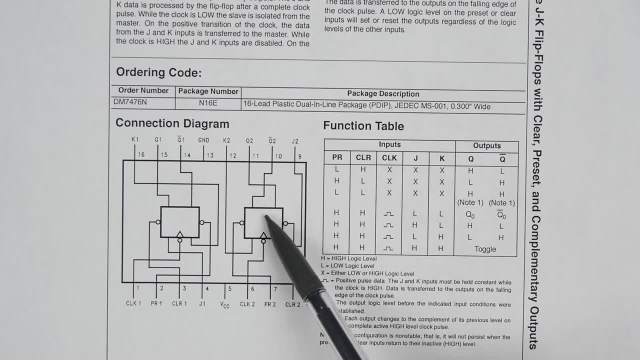 But in this case I've got the 74LS76, and you can see it's got two JK flip-flops in it. If we just look at one of them, you've got the output. so there's the Q output, and then the Q inverted output, and then, of course, you have the J input. 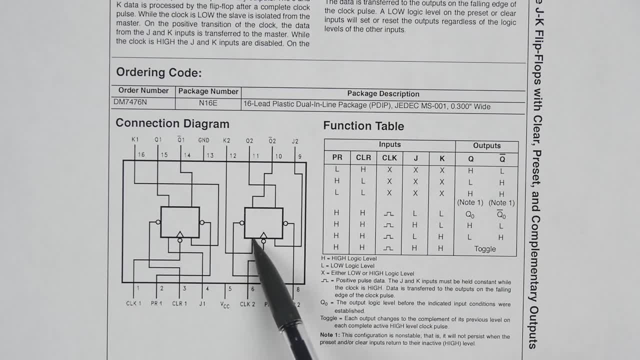 And the K input. somewhere here it is K input. So you've got the J and K input and then the two outputs, the Q and the inverted Q. We've also got the clock input here, which of course we want, and you can see it's an inverted clock. 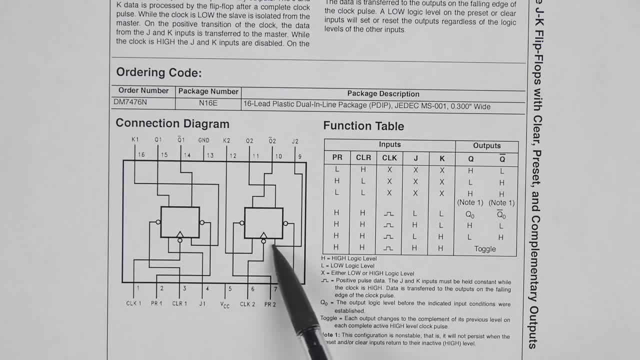 which means that this is going to switch states on the falling edge of the clock, which doesn't make a big difference, but it does mean, you know, just, we should expect to see that the state change on the falling edge and they show the whole clock signal here, because I think what they're implying is. 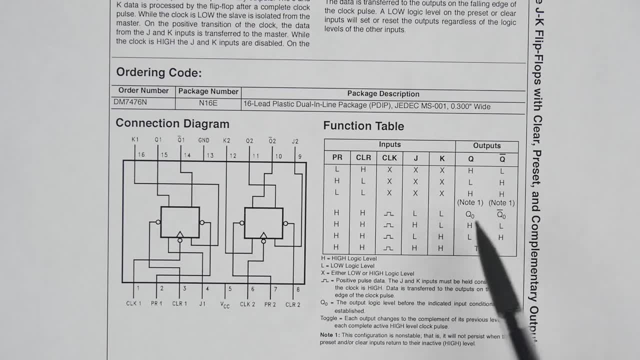 that you know. after a complete clock signal then it changes state And this also has a preset and a clear input, and so preset and clear are basically a way to ignore the clock and just set the output So they're active low. You can see the little bubble here is telling us they're active low, So normally they'd be high, preset and clear. 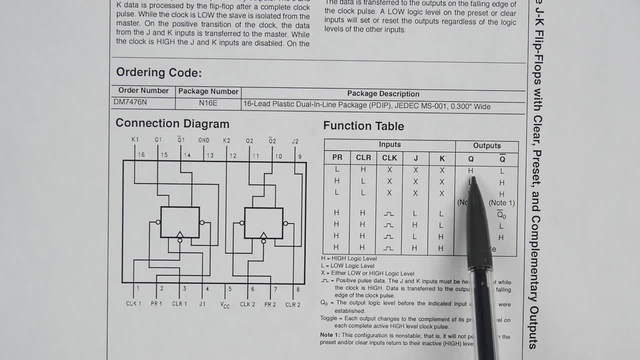 but if you take preset low then that forces the Q output high, regardless of what's going on with the clock Or the J and K inputs. So it's just kind of an override to preset the output And then clear is the same thing If you take that low. 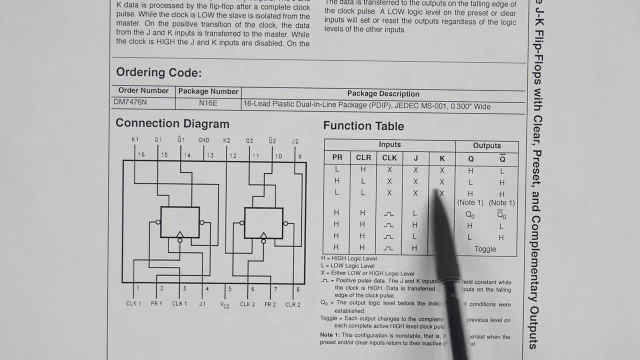 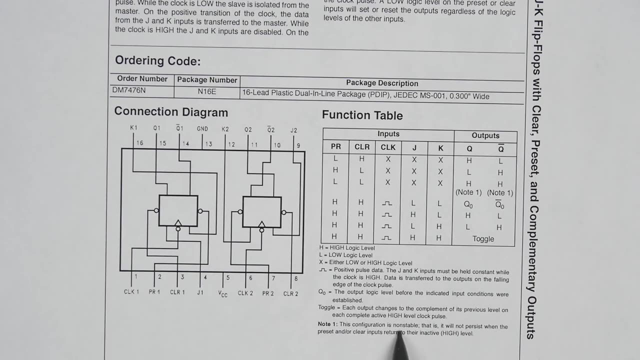 then it forces the output low again, regardless of what the clock or J or K inputs are doing. And then you know, if both preset and clear are low, then both the outputs go high and that's kind of an invalid state. And in fact they have a little note for us here. It says: note: this configuration is non-stable. 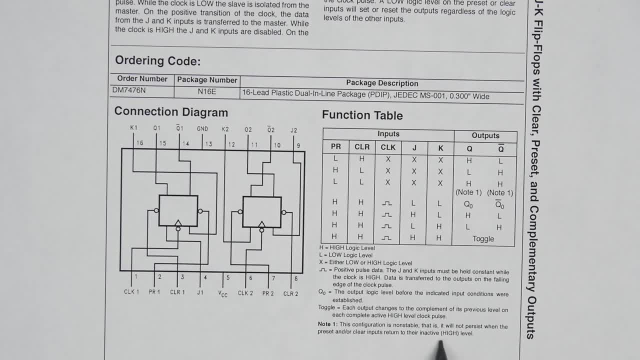 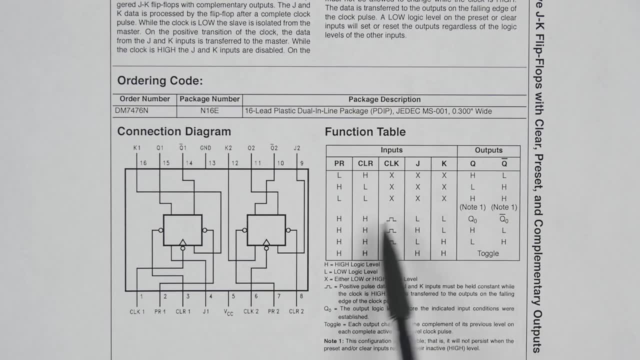 That is, it will not persist when the preset and or clear inputs are active, Return to their inactive high level. So basically they're telling us: don't, don't do that. But this is just kind of an override kind of thing. 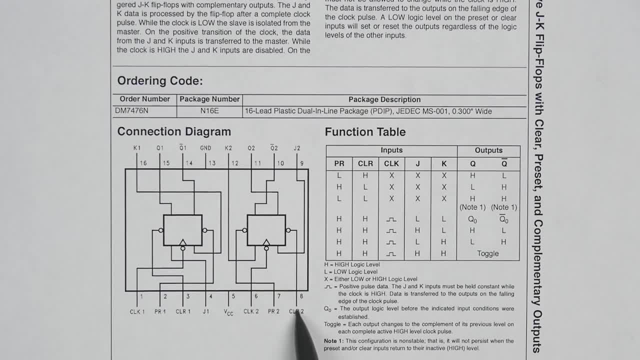 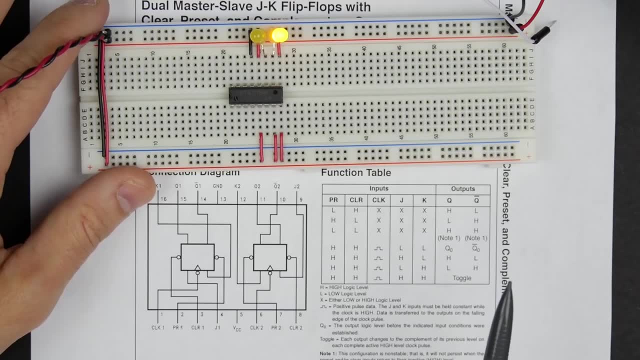 So we'll set both of those high so that they're not being used. And so I've set this circuit up using this chip and you can kind of let me see if I can fit it all in here. But you can see, of course we've got VCC and ground to provide power to our chip. 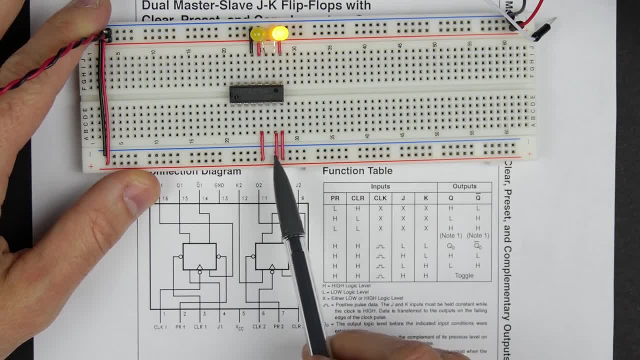 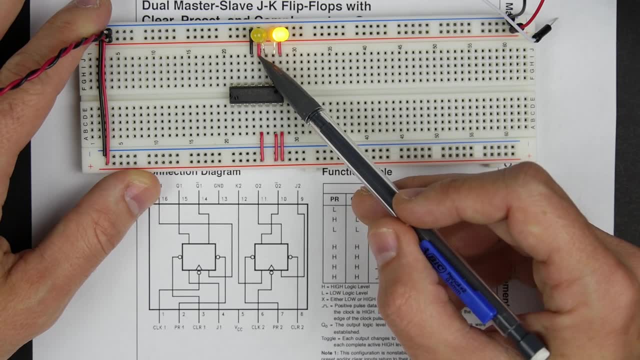 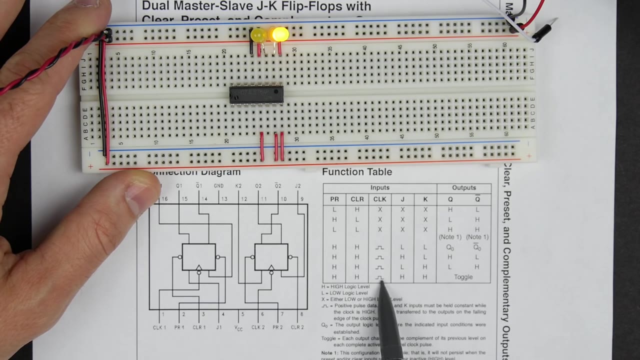 So those are hooked up there And then the preset and clear are both high, which is they're inactive. And then you can also see I've got the J and the K inputs are set high. So basically I'm inputting a high and high to the J and K, which means that when our clock pulse comes we'll toggle. 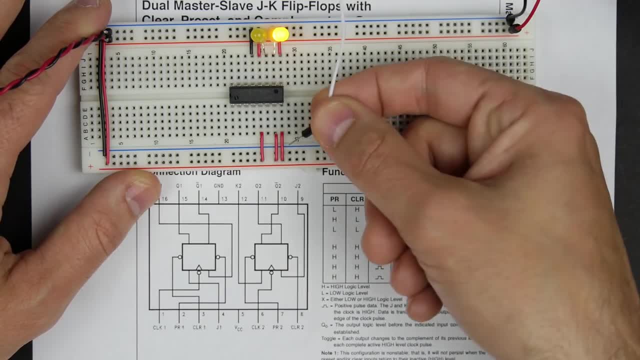 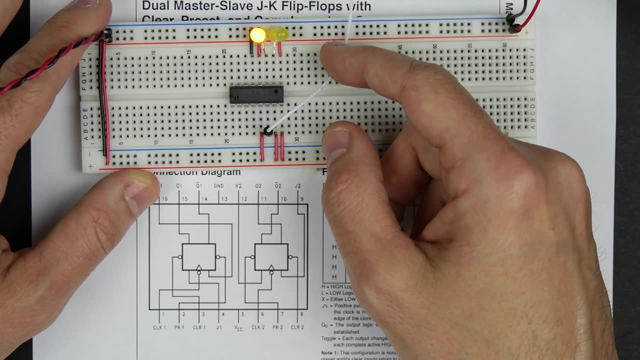 And you can see the two outputs. So I connect the clock up to our clock, which is pin six. here You can see it's toggling with each clock pulse And so if we look at it together with the clock you can see it's toggling. 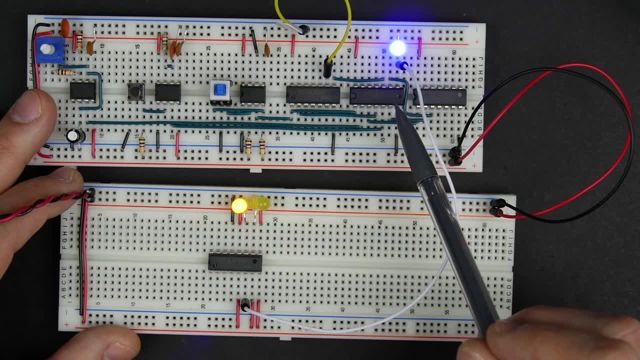 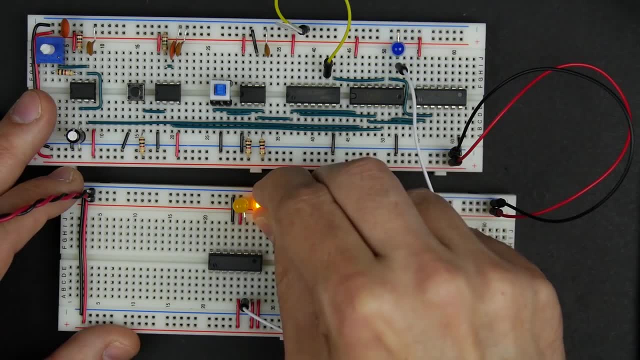 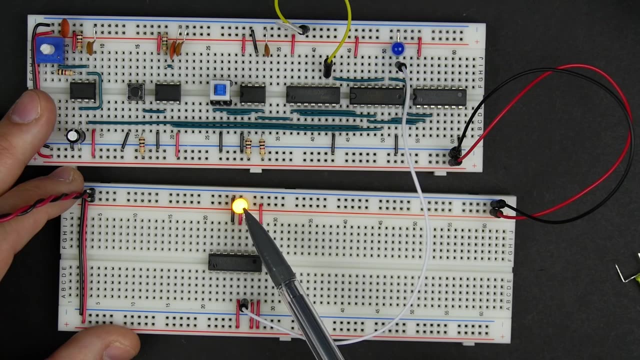 toggling each time the clock is pulsing. Now, an interesting side effect here is, if I it's kinda easier to see if I take out the inverted Q output, but an interesting side effect here is that you can see the output is toggling. 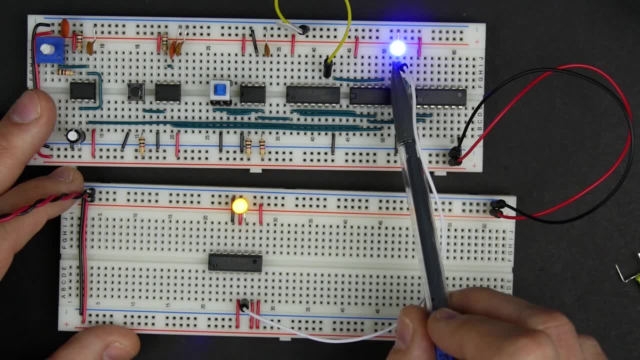 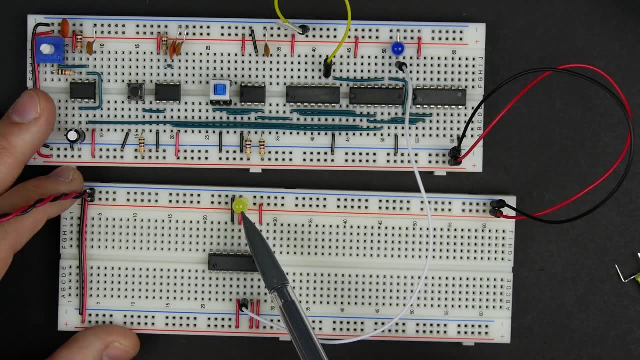 at half the speed of the clock, And so this circuit is sometimes referred to as a divide by two, because whatever speed the clock is coming in, the output here is that speed divided by two, And that can get kinda interesting if we keep dividing by two. 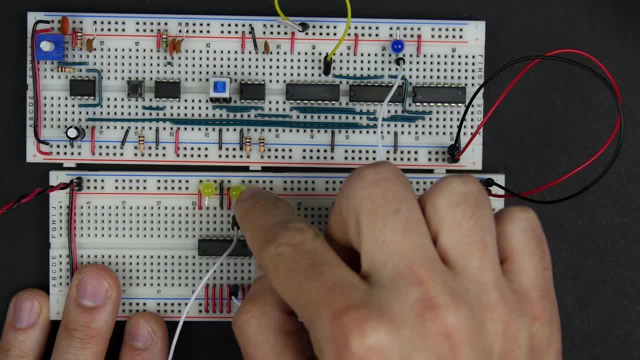 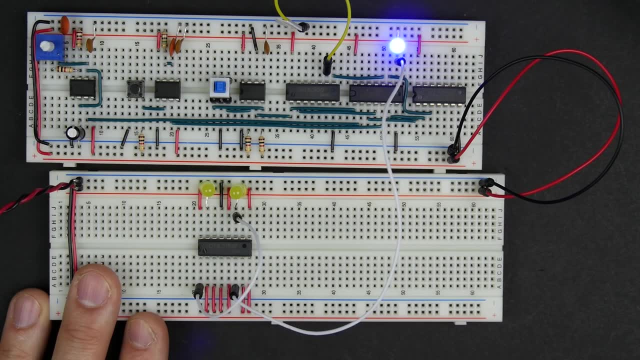 So if we take the output of the first flip-flop and we use that as the clock for another flip-flop, we see that now this second flip-flop is toggling at half the speed of the first, which is toggling at half the speed of our clock. 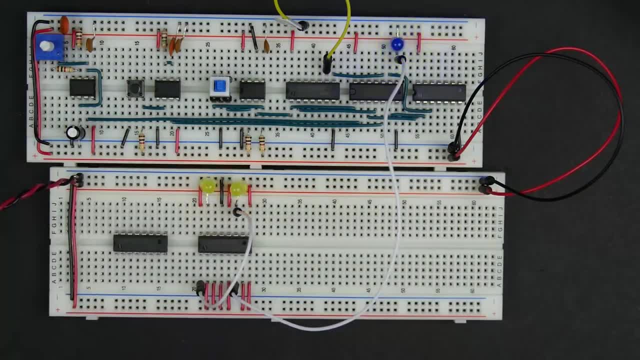 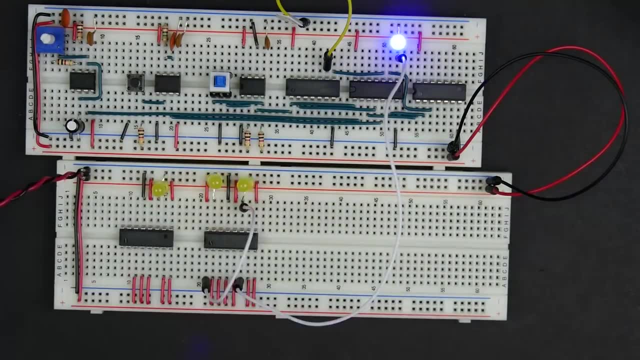 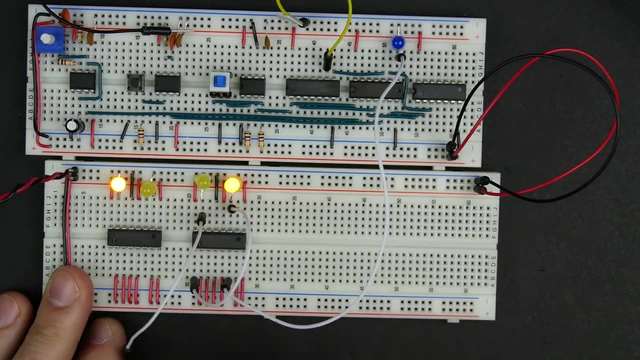 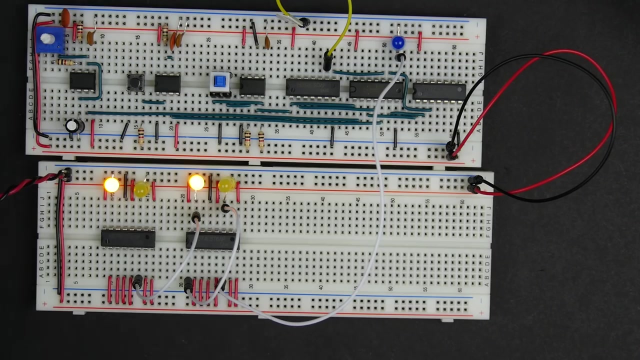 And of course we can keep going. So now, if we hook up two more of these, we can take the output of this one and feed it into the clock of the next one, And then we can take the output of the next one and feed it into the clock of the next one. 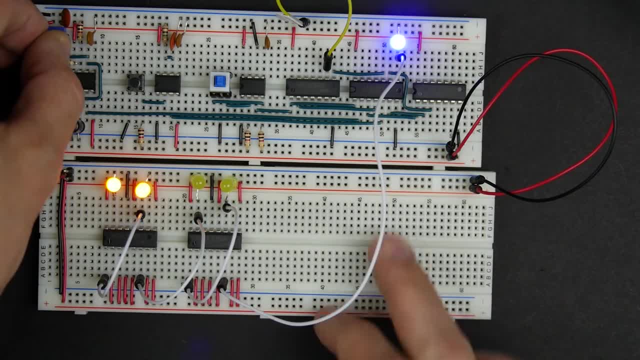 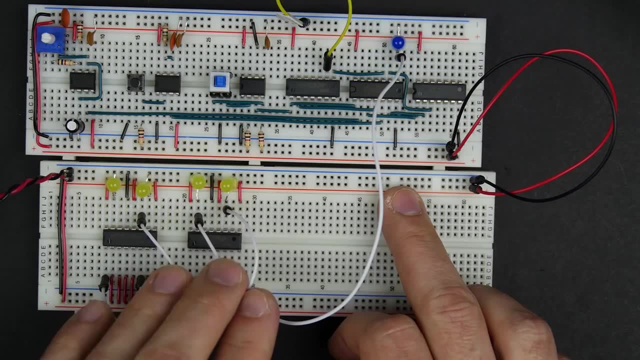 And if I increase the speed of the clock a little bit, you'll see something interesting that's happening here, Because we're dividing by two each time, what we've got is a binary counter: Zero, one, two, three, four, five, six, seven. 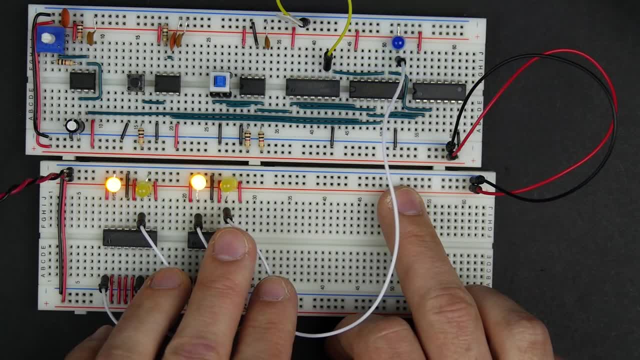 eight, nine, 10,, 11,, 12,, 13,, 14, 15.. It's counting in binary. So now we've got a binary counter.